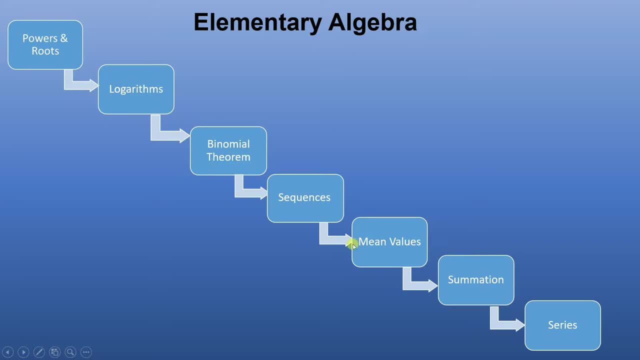 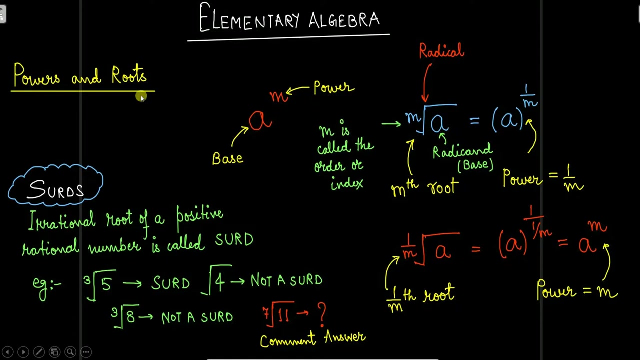 and roots. logarithms, binomial theorem, sequences mean values, summation and series. Okay, so I hope you got a clear idea what will be the order of the lectures that will be getting uploaded. So the first topic that we're going to see is powers and roots. So this: powers and roots. 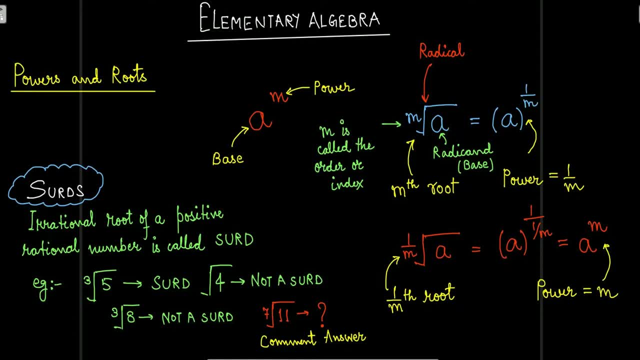 just focus on this pointer and whatever I am speaking. Okay, so listen this, listen my voice carefully and just see this pointer. Don't see whatever is written on the board at once. Okay, if you listen my words carefully and if you see this pointer, I assure you you'll get a very good. 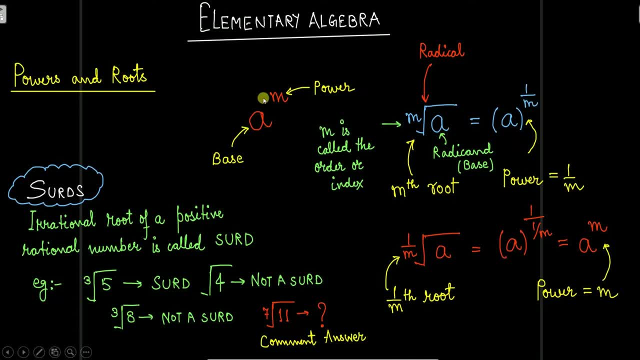 grip on the command or command on the subject. Okay, now if this could be written. and now see what is written here: this is a to the power of m. What is a? This is called as the base and m is called as the power. Okay, now this: if something is written like this, that is mth root of a. So how? 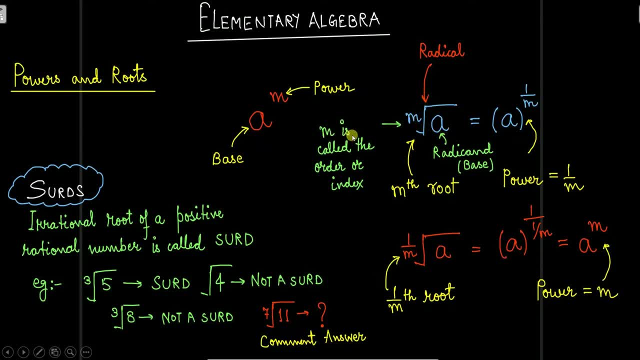 will you read this? This is read as mth root of a. So what is m? m is called the order or the index, m is called the order. Now, this symbol, as you can see, this symbol is called as the radical, and whatever is written, 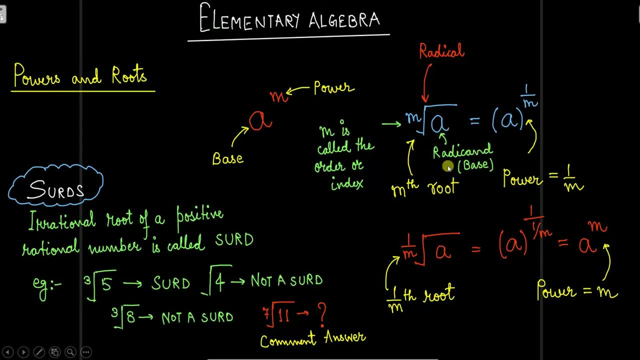 inside this radical, so that is called as a radicand or base. Okay, so r-a-d-i-c-a-n-d. radicand or base. Now this could be read as mth root of a. Now. another way of representing this is: you can. 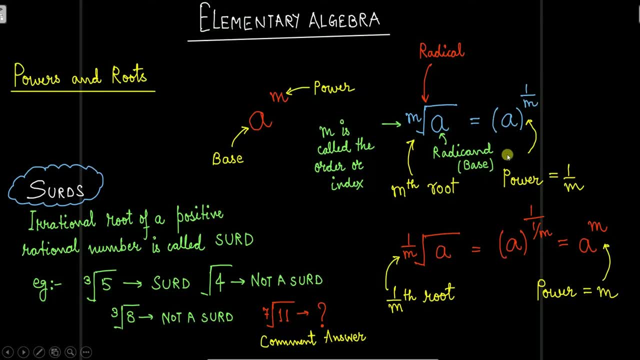 write this as a to the power of 1 by m. You can write this as a to the power of 1 by m, All right now, instead of m. if you write 1 upon m, So this could be written as a to the power of 1 upon 1 by m is equal to a to the power of m. What is the rule? 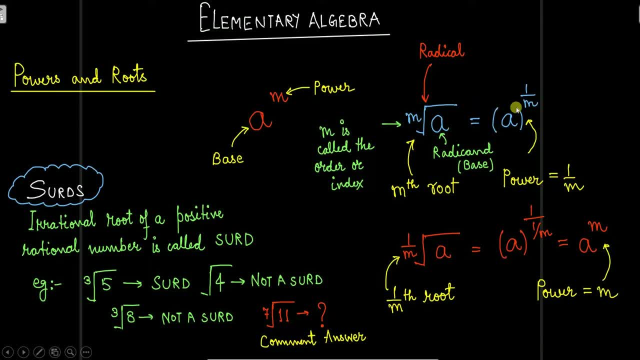 Now see whatever is written on the left hand side. if you write this in the format of something raised to the power, so that thing will be coming under the denominator and the numerator will always be 1.. Okay, so if here it is p, so this could be written as a to the power of p. If here you are. 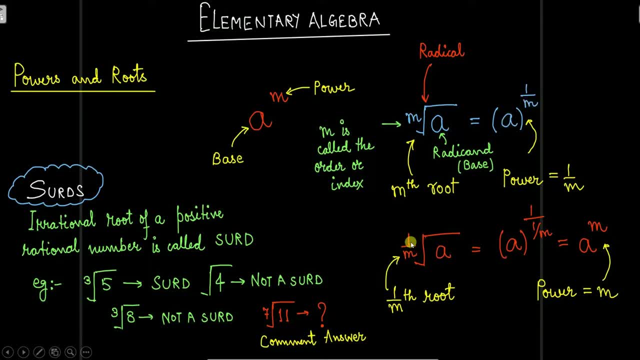 writing 3, so this will be a to the power of 1 by 3.. If here you are writing 1 by m, so here it will be a upon 1 upon 1 by m. So this is again a to the power of m. Why? Because m will come over. 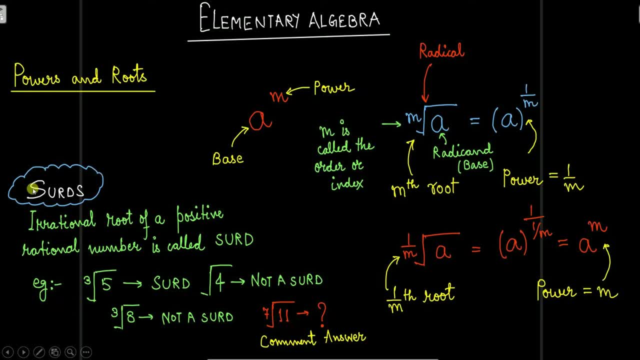 Now you might be, you might have come across this word called certs. So how will you define this cert? So certs are nothing but the irrational root of a positive rational number. So what is a cert? Irrational root of a positive rational number. So what is 5?? 5 is a positive rational number. Okay, 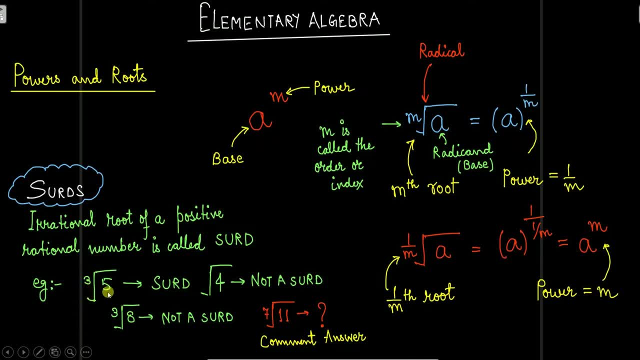 it is an irrational root. that means: just see this example. Will you get any whole number value for this? No, you won't be getting any whole number value for this. If you just type this in calculator and get this value, you will get in some decimal values. Okay, so this is not a rational number. 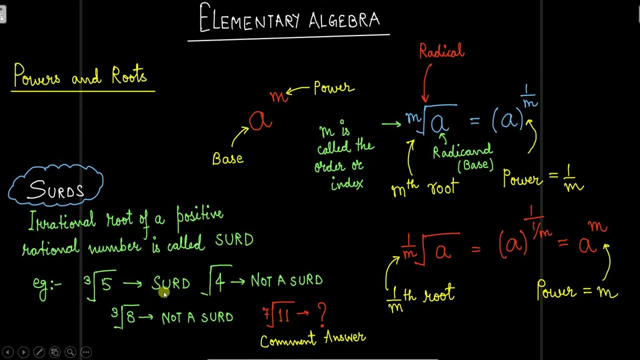 So now, since this, our solution, is not a rational number, so that is why this is called a cert. Okay now if this is written as 4.. Okay now, what is here if anything is not, if anything is missing here, what does it mean? Just remember: if anything is missing here, what does it mean If anything is? 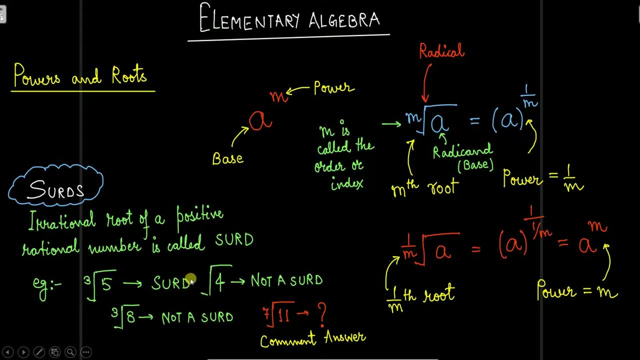 missing here it means 2.. If anything is missing here, it means 2.. Okay, so this could be written as 4 to the power of 1 upon 2.. Okay now, square root of 4 is 2.. So 2 is a whole number. So that means. 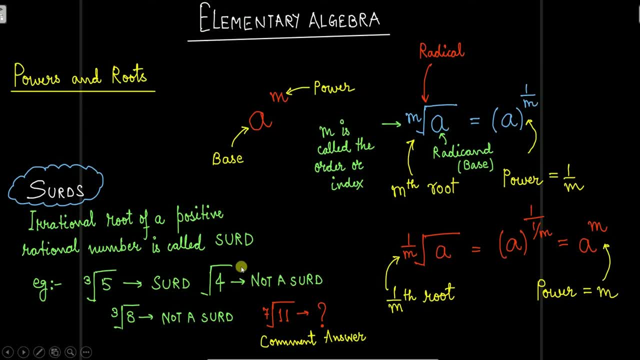 it is not an irrational number and hence it is not a cert. I hope this is clear to you. Moving to third example Now, this is cube root of 8.. Can you call this as a cert? No, we cannot call this as a cert because 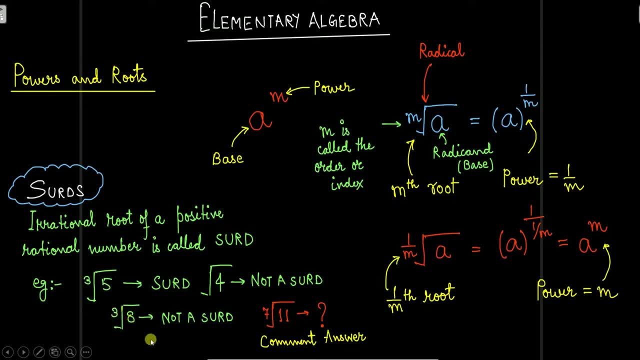 if we find this cube root of 8, we will be getting the value as 2.. So that is why 2 is a whole number and hence it is not a cert. Now one question for you: 7th root of 11.. Now tell me, comment your. 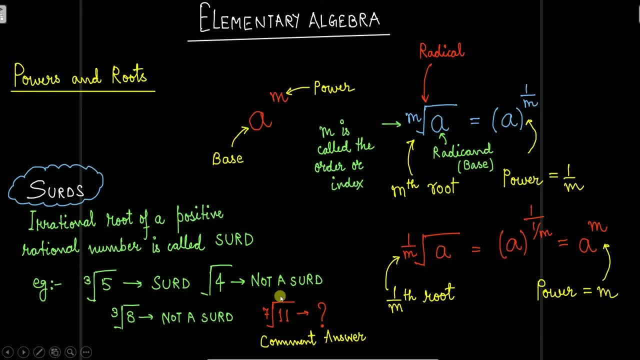 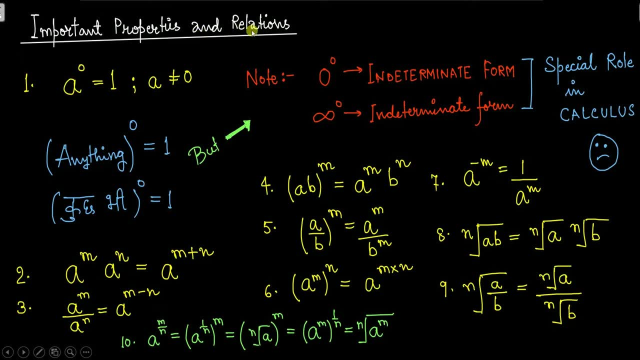 answer in the comment box whether this is a cert or whether this is not a cert. Okay, now there are some important properties and relations of powers and roots. Okay, so the first property that we know is a to the power of 0 is equal to 0. So this is a power of 0. So this is a power of 0. So this is. 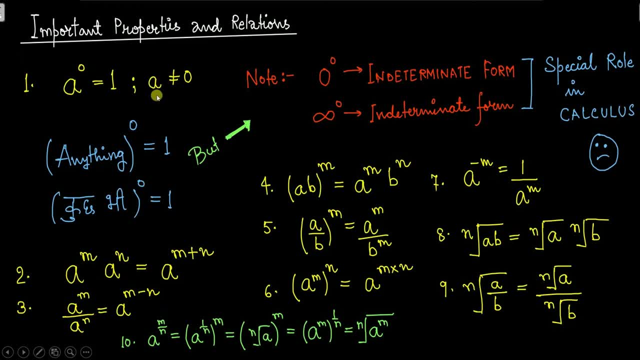 a to the power of 1 or a raised to the power of 0 is equal to 1, provided your a should not be a 0. Now if a becomes 0, so that will become 0 to the power of 0. That will become an indeterminate. 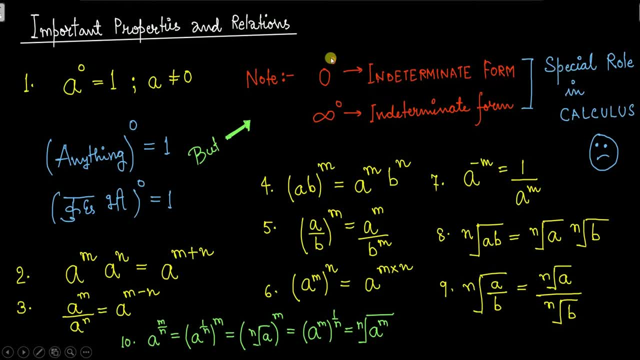 form: Okay, so these things we will be seeing in calculus. So these are the special, these have some special rules in calculus. these forms: Okay now. anything raised to the power of 0 becomes 1.. Anything raised to the power of 0 becomes 1.. So if your name is Govind and Govind is raised to the 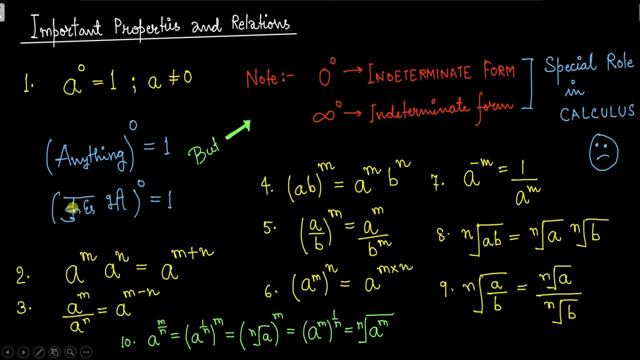 of zero, so govind will get converted into one. okay, so whatever you write. so this is written in hindi, it's written- could be anything. anything raised to the power of zero will give you one, but there are some special cases. so you will be asking, sir, instead of anything, if i write infinity. so 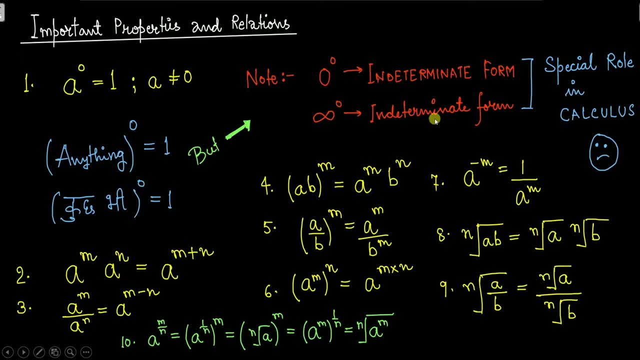 what does it infinity means? so infinity to the power of zero is an indeterminate form. remember, infinity to the power of 0 is an indeterminate form. okay, so here they have got some special roles in calculus here simply the way of representing this infinity. okay, now what? 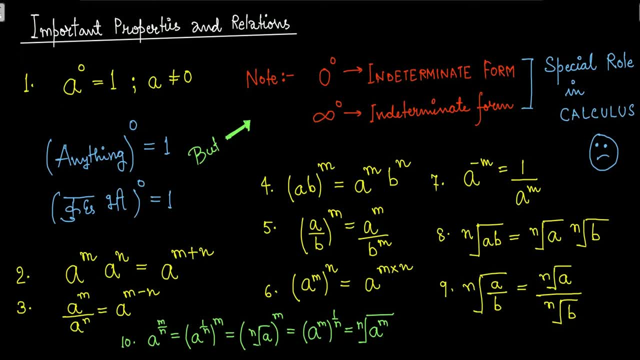 is it infinity? does it infinity actually means anything? infinity means any, any, any value which is much, much, much greater or higher than anything. okay, so obviously you will be putting some any finite value, isn't it? so any finite value to the power of zero will give you one, but if any, 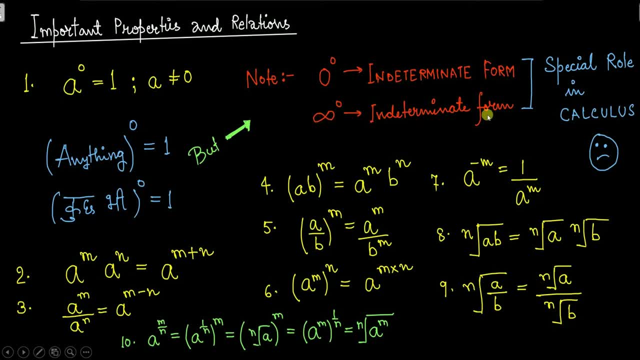 inf passé is finite value, then you should be drawing. thank you��는 one. but if any infinite value to the power of zero will give you one. but if any infinite value you will be drawing, value is there which is raised to the power of zero, that will become an indeterminate form. so 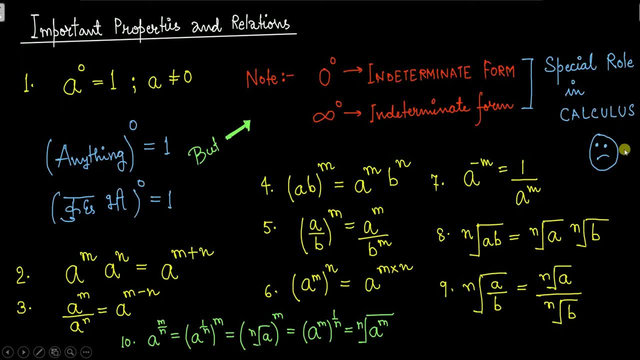 remember these two things have got some special roles in calculators. okay, so this is the first property. remember this. coming to second property, second property says a to the power of m, a to the power of n will give you a to the power of m plus n. so why i have added this? because the base is: 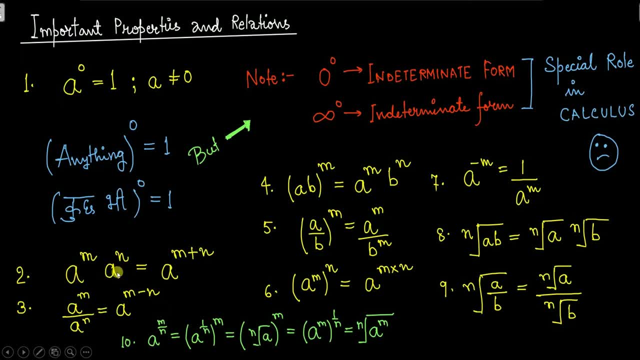 same. here is also a, here is also a. so whenever the base is same, the powers gets added, the power gets added. remember: this third property says a to the power of m. a to divide upon a to the power of n will give you a to the power of m minus n. all right, so this is when the powers are, when the 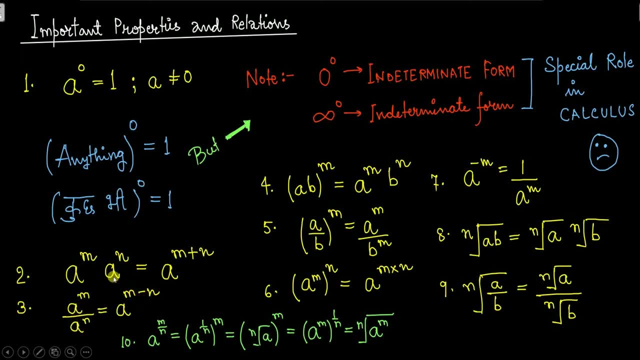 base is same and they are divided. so the powers are subtracted when the base is same, and when they are multiplied, the powers are added, and when the base is same, the powers are divided, and when they are divided, the powers are subtracted. so i hope. first, property, second: 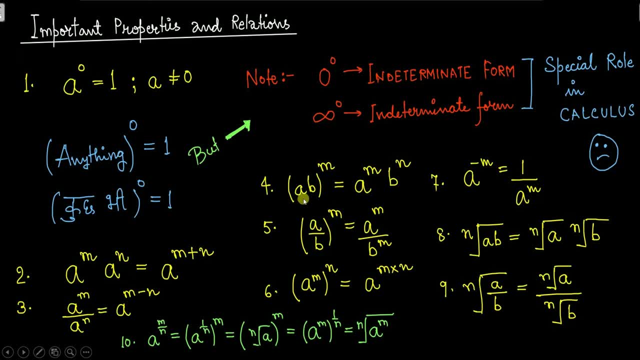 property. third property is clear to you. moving to fourth property, so if a- b is raised to the power of m, the product of a- b is raised to the power of m. so what is the rule? that whatever is written in the power, that will get distributed in each of the two values. okay, so each of the two variables. 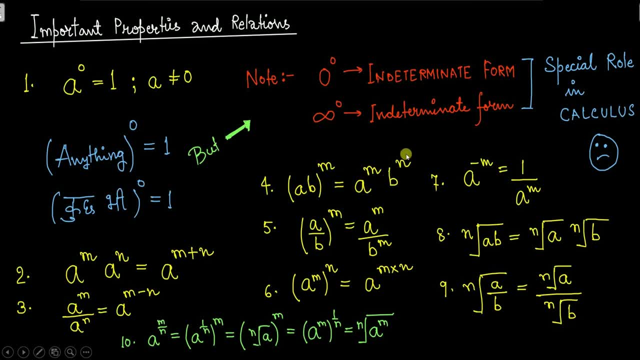 so a to the power of m and b to the power of m. sorry, here there is some mistake. it will be m. okay, so that's a typo error, sorry for that. so a, b to the power of m will give you a to the power of m into b to the power of m. okay, now point number five. point number five: we have a by b to the power. 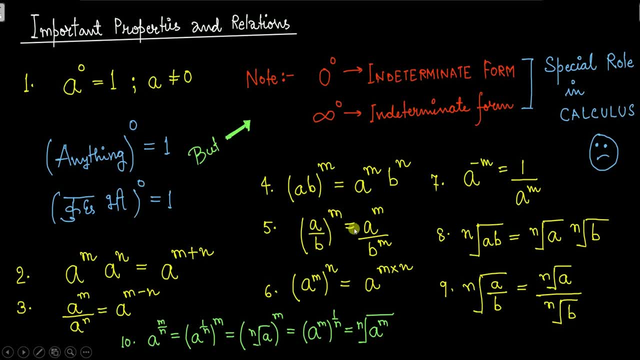 of m. so here also m will get distributed upon this a and b. so this could be written as a to the power of m divided by b to the power of m. okay, now, sixth property. we have a to the power of m, whole to the power of n. will give you a to the power of m. 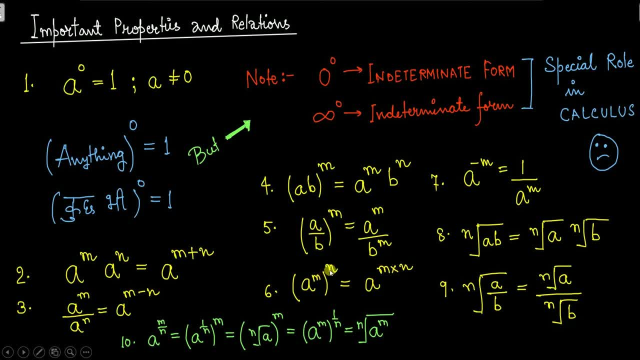 cross n. m cross n means these two. these two values are multiplied, so a to the power of m into m whole to the power of n will give you a to the power of m into n. moving to the seventh one that we have is a to the power of minus m, so this could be written as one upon 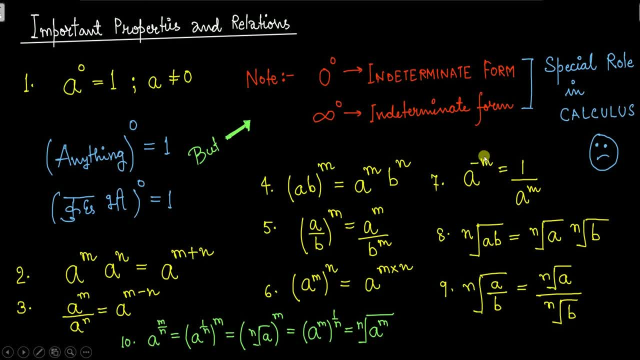 a to the power of m. okay, so whenever you find anything written raised to the power of minus, so that makes this factor to come in the denominator. okay, so a raised to the power of minus m will give you one upon a to the power of m. eighth property. let's see. so just now we have 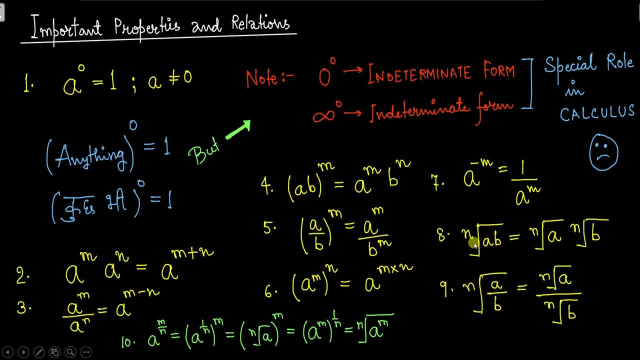 learned. how will you read this? this could be read as nth root of a- b. this could be read as nth root of a- b. now, since this is written as nth root of a- b and here a and b are products, so this nth root could be distributed in each of the two variables. that is, nth root of a multiplied with nth root of. 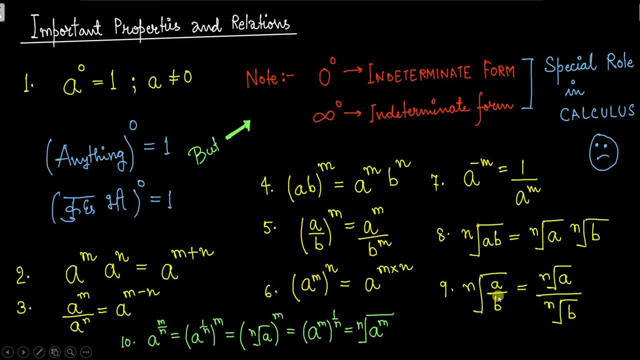 b. coming to the ninth property, nth root of a upon b will give you nth root of a divided by nth root of b. okay now, similarly, same rule. if the product is multiplied, so the factors get separated and they are multiplied. and if it is divided, whatever is, if the radicand is is a division of two, number, that is, it's a fraction. so the this nth factor, or